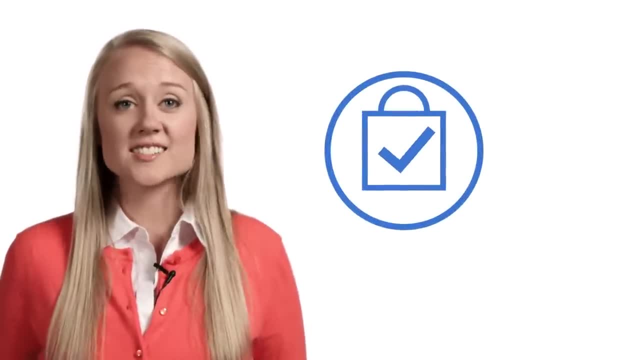 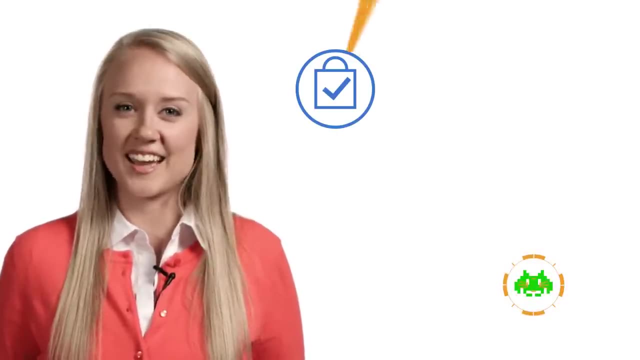 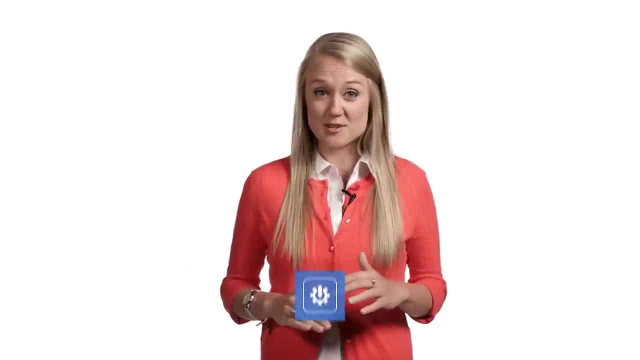 protection service like SiteLock Security. SiteLock scours your site for malware daily and automatically removes it, saving you time and worry and protecting your site against hackers too. Fourth, frequently update your applications and plugins. Now, this is absolutely critical for preventing. hacker attacks. Running old software is like driving a car with an open recall for catching on fire. You're just asking for trouble. Security holes are constantly being remedied each time new software is released. If you have any questions, please feel free to reach out to me at. 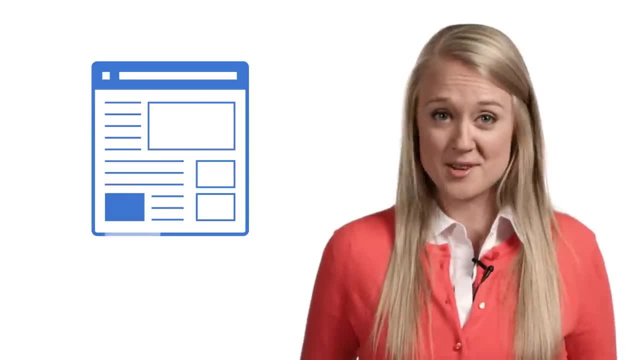 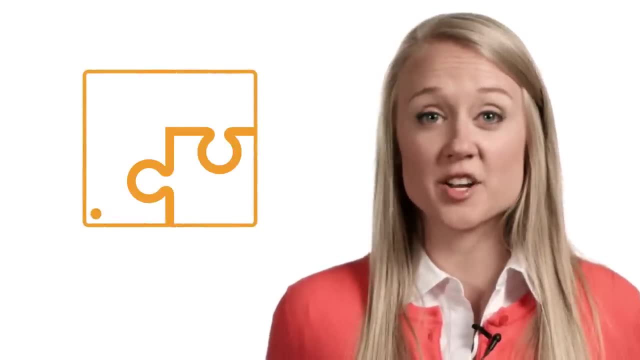 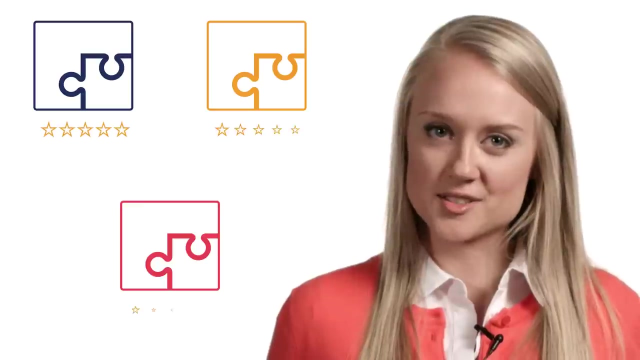 sitelocksecuritycom and I'll be happy to answer any questions you may have, And this applies to plugins too. If you subscribe to a plugin security announcement list, you'll never miss an opportunity to update. Just keep in mind that not all plugins are created equal, so only install those that are highly 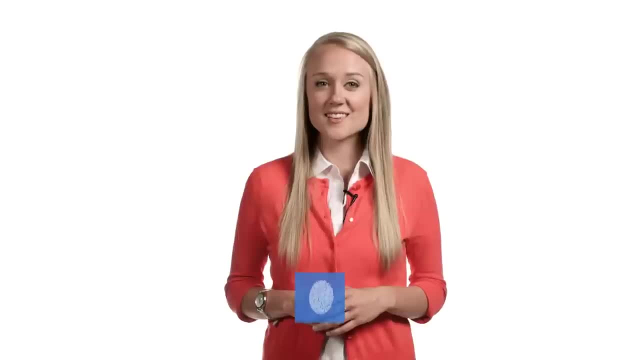 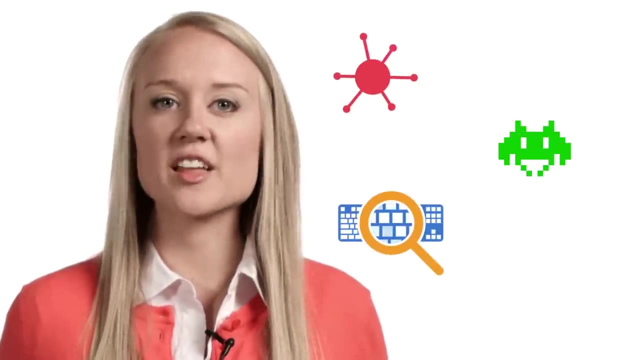 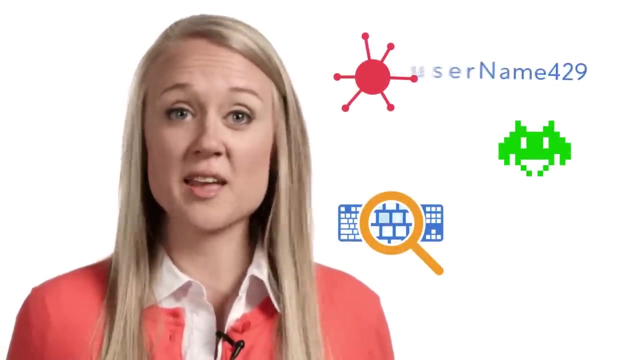 reviewed and have a reputation as being safe. Fifth, access your site only from secure locations. Viruses, malware and key loggers, which is surveillance software that records what you type, can be discreetly installed on computers by hackers and used to obtain your username, password, credentials or even infect your 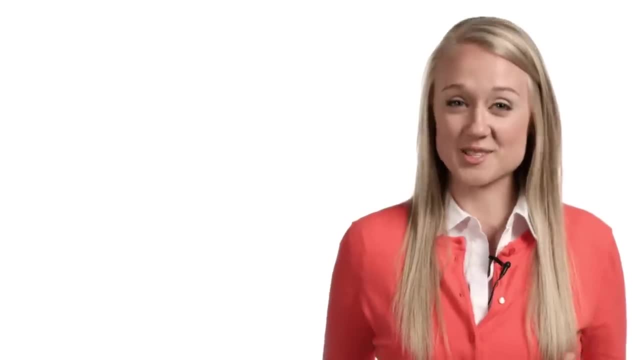 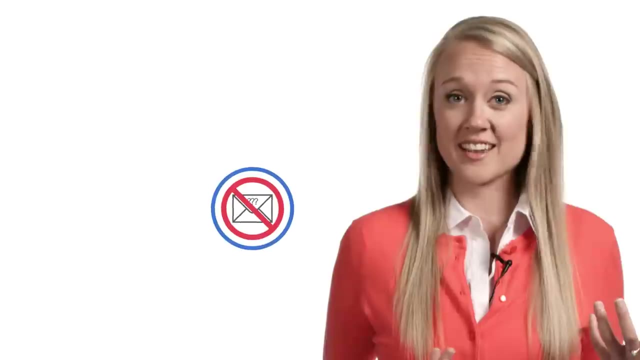 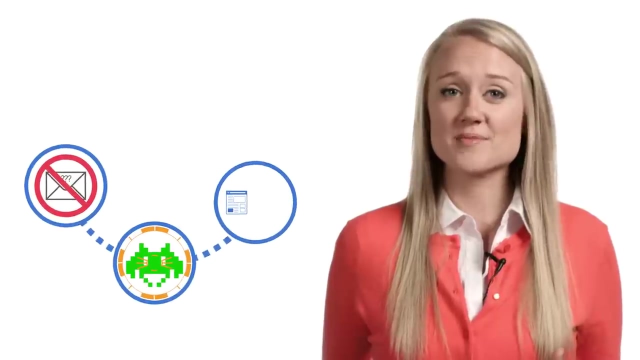 website files themselves. Practicing good at-home security means taking common sense measures such as never opening emails or attachments from people you don't recognize, using a reliable antivirus or spyware scanner, backing up your website and database frequently, avoiding rogue websites and just being careful. 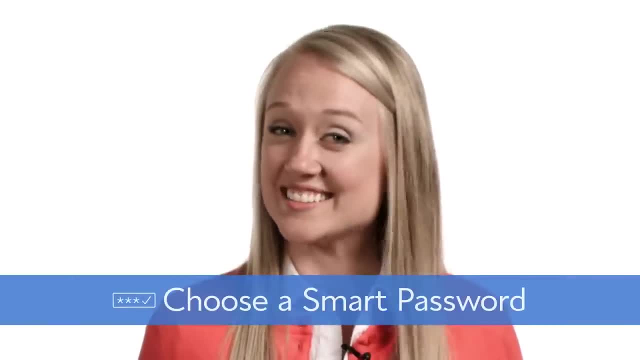 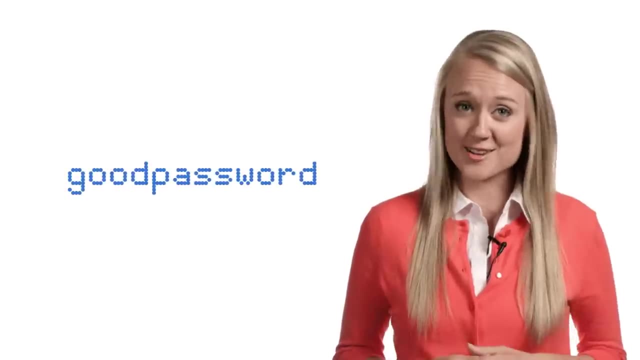 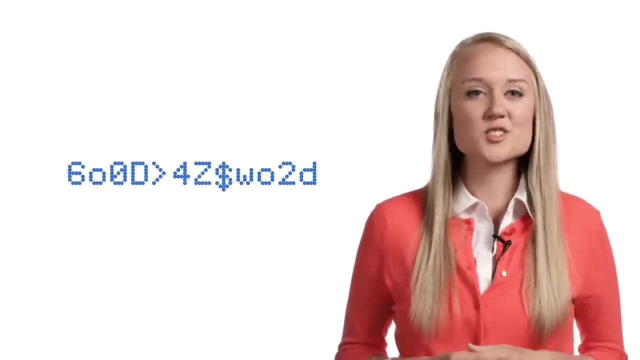 about where you share your information. Last but not least, simply choose a smart password. Smart passwords are long, a minimum of 12 characters to be exact. They should also use a combination of numbers, symbols, upper and lower case letters too, And you shouldn't rely on the same password you use for your email. 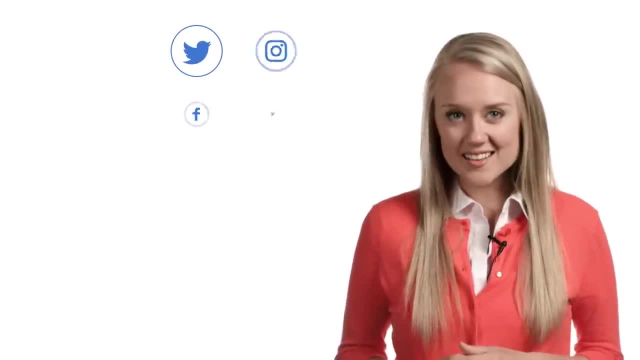 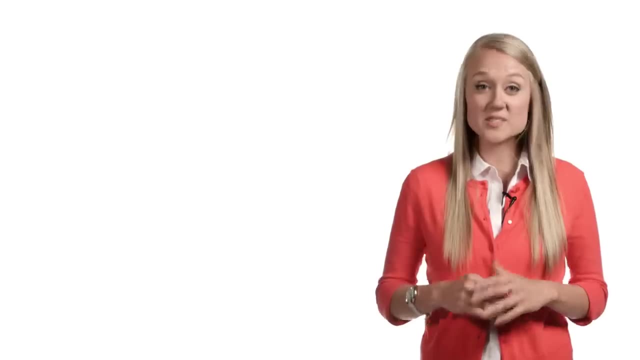 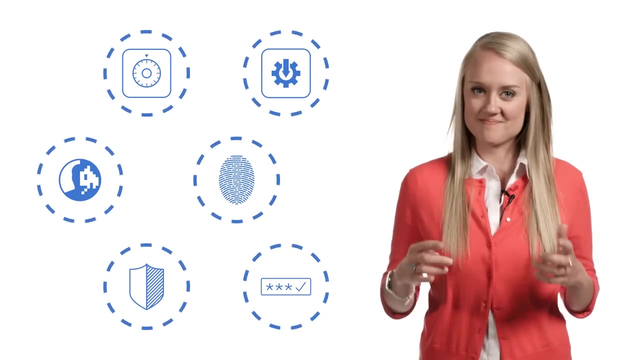 or social media accounts, Make sure to make it unique and complicated. A little preemptive site security can save you from huge headaches down the road. So take a moment, review these six tips we just covered and ask yourself: am I doing everything I can to protect my website now? If not, start today And if? 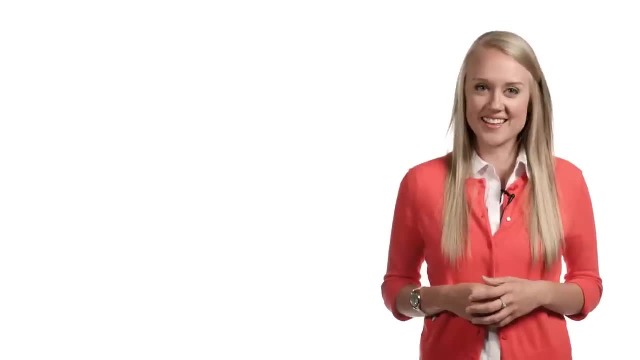 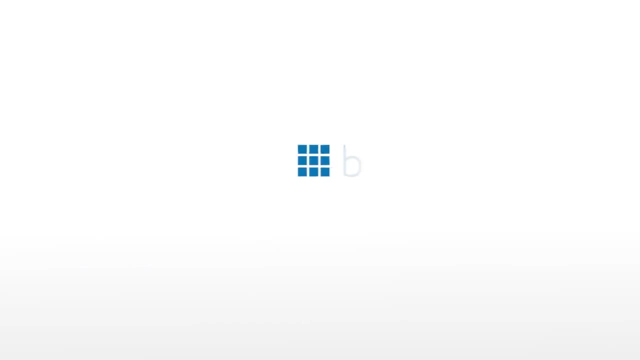 you need a little help. Bluehost experts are standing by. Give us a call at any time and we'll help you give your website the absolute protection it deserves.